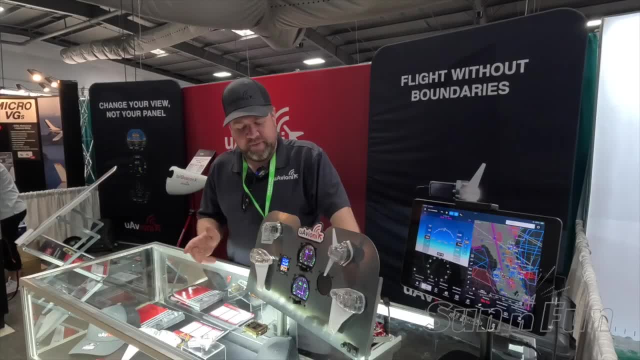 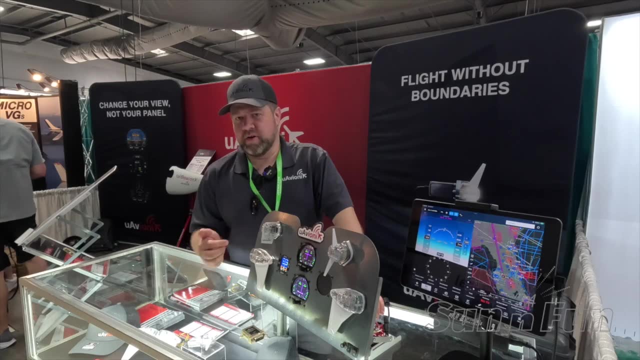 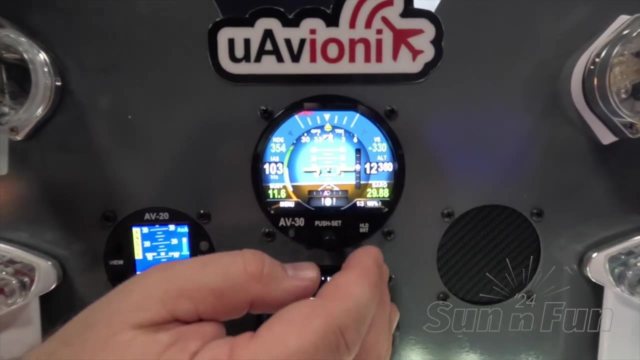 provide VFR-only guidance. The AVHSI adds interface for IFR navigators, both GPS and VOR. With it we added several new modes to the AV30 that can display it. We can display vertical and lateral guidance on the attitude indicator on an HSI display. We have an overview map view. 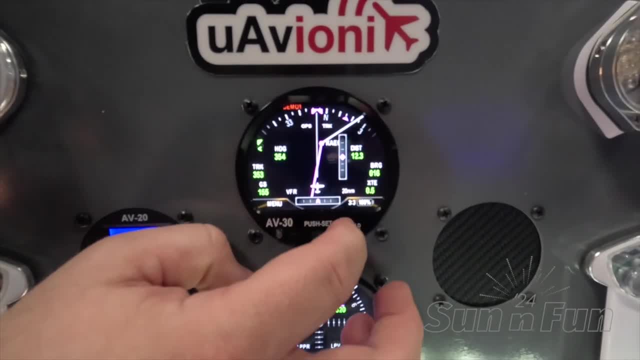 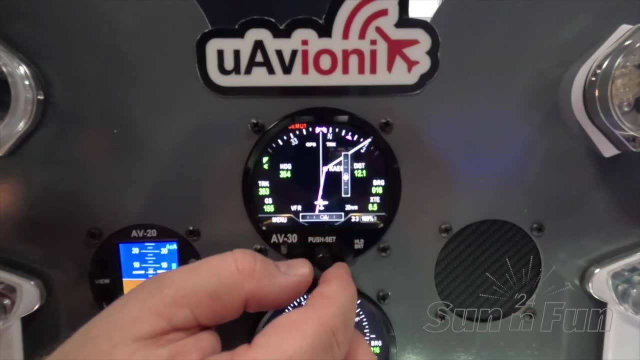 as well as a traditional CDI view. The AVHSI also synchronizes data between multiple AV30s. You can have up to four AV30s connected to one AVHSI and sync that data. So if you set heading bug on one, it'll set on all of them. If you set barrow on one, it'll set on all of them. 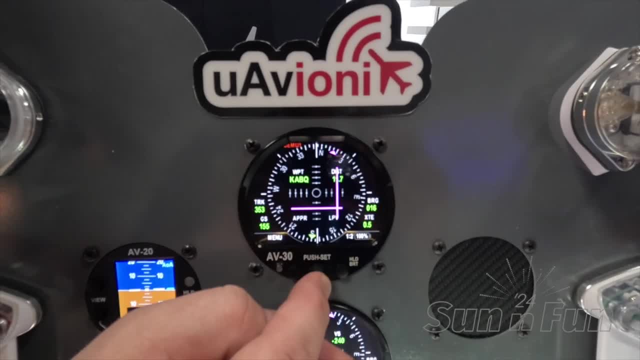 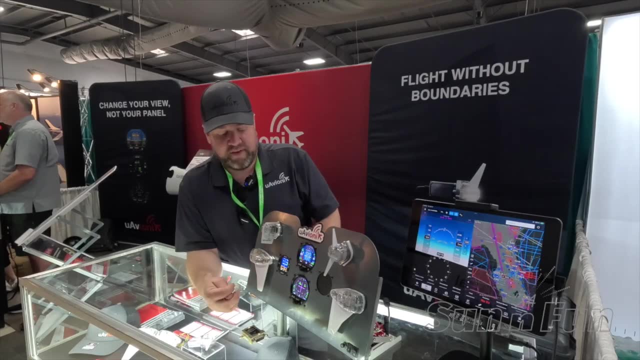 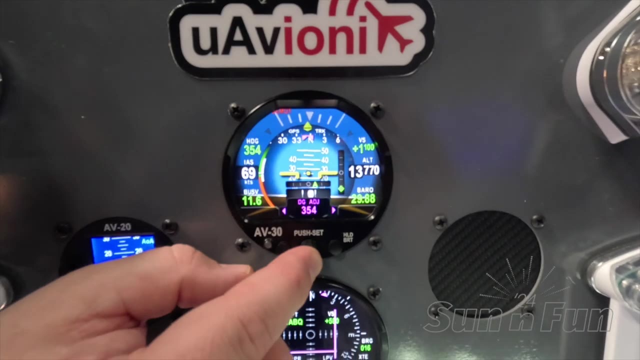 really making it a streamlined solution for especially single-pilot IFR in your high workload environments. Walking through the screens of the AV30 with the AVHSI, first thing on the attitude indicator you'll notice is there's both lateral and vertical guidance That'll display for both GPS approaches as well as an ILS approach On the HSI display. 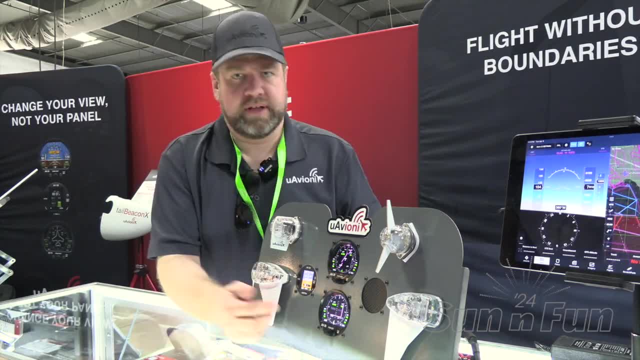 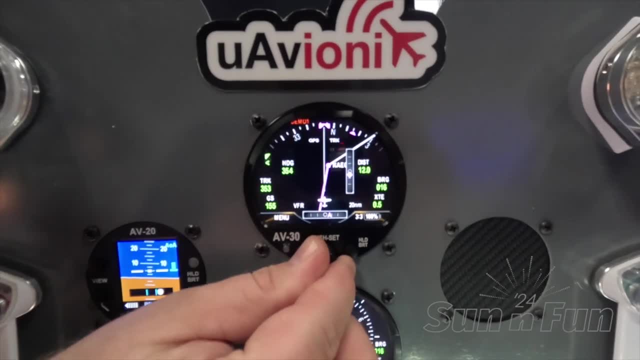 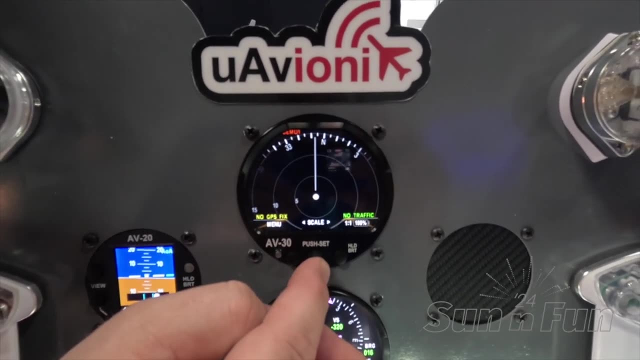 this will look familiar to AV30. users, but we've added the vertical guidance. That vertical guidance will show up automatically when you're on an approach or getting a glide slope from an ILS. Additionally, the AV30 has always had the ability to show flight plan to the next leg. We've added additional capability here. 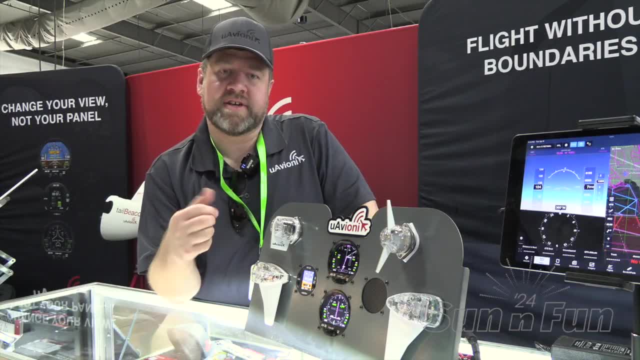 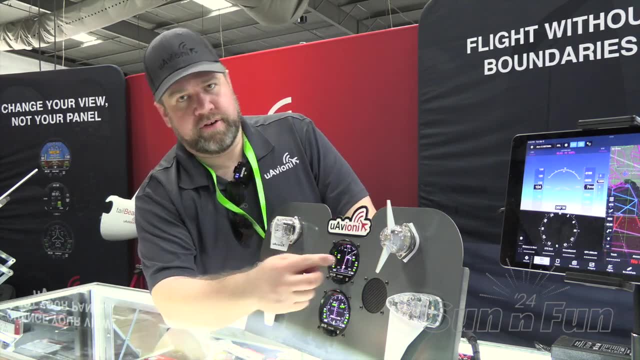 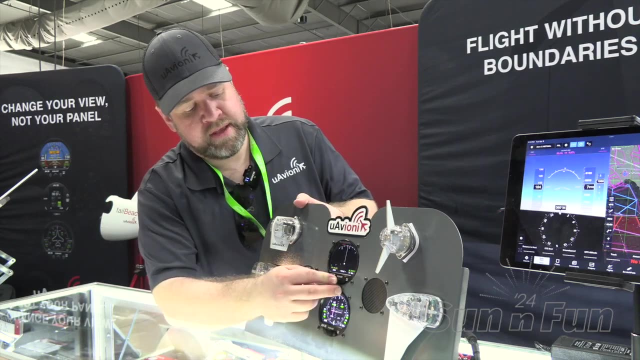 where it'll show a full flight plan. It'll also show curved flight plan legs, So if you're flying a DME arc or a holding pattern, it'll show up right here. Lateral and vertical guidance also available on this screen. We've also added a阿V link with Savior tracks. See that. 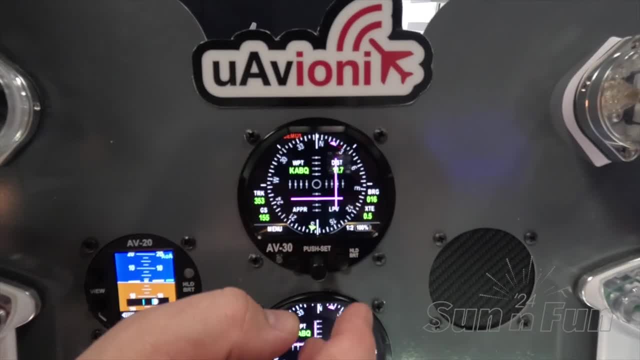 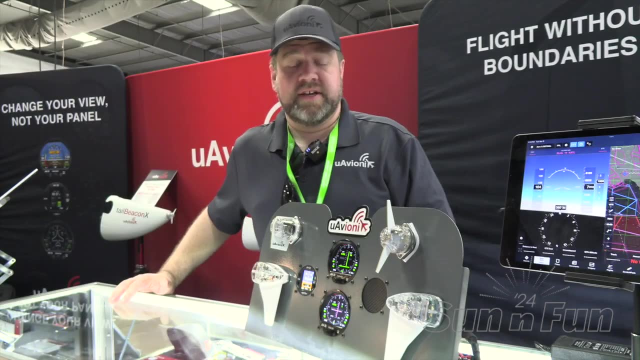 There's our traffic display page if we had an av link connected. And here's the CDI view. that'll look common to you know, pilots like me that flew with the traditional mechanical CDI. The AVHSI is available now for experimental aircraft. 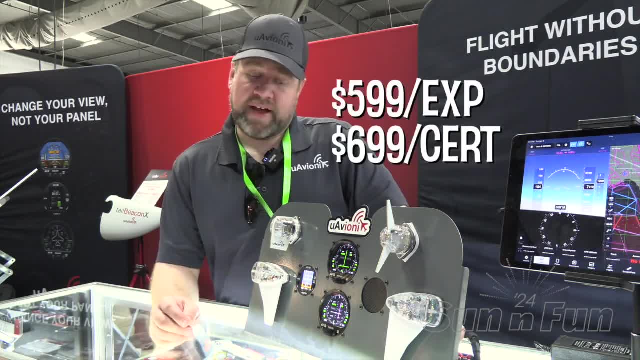 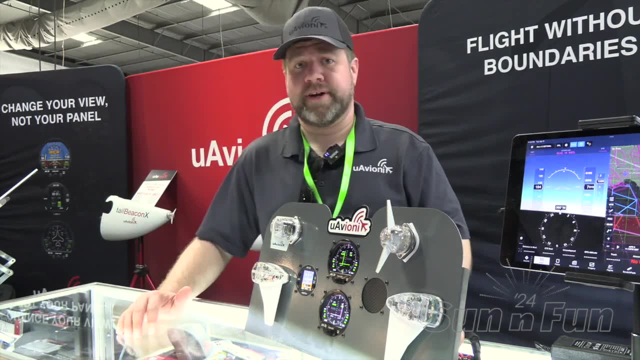 We rolled it out here at Sun and Fun and it'll be shipping within the next few days. It's $599- $599 right now. It'll be available for certified aircraft And it'll be $699 at that point for certified.